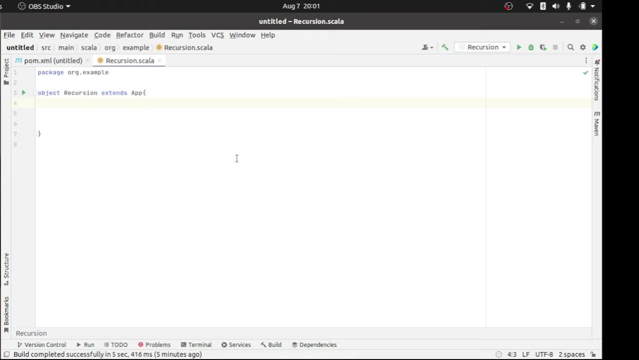 a normal recursion function. So let's start our video. So first I will be doing a hands-on in the recursion, like how to write a recursive function. We will be writing the normal recursive function and a very good example of it: the factorial. 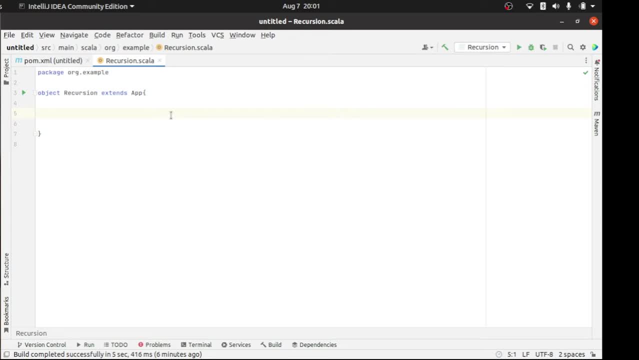 of a number. We will be doing the factorial of a number, So let's start writing factorial of a number. This is our tail recursion. So let's start writing the factorial of a number. This is our tail recursion. So let's get back to our. 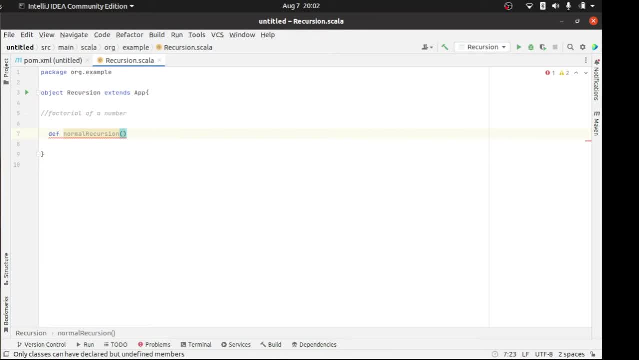 table. So back in scala you're going to have to really think about how in Scala you will be writing the total recursion investigative function. shall we adjust a little bit here of big integer type. why I am giving this value as big integer you will learn in. 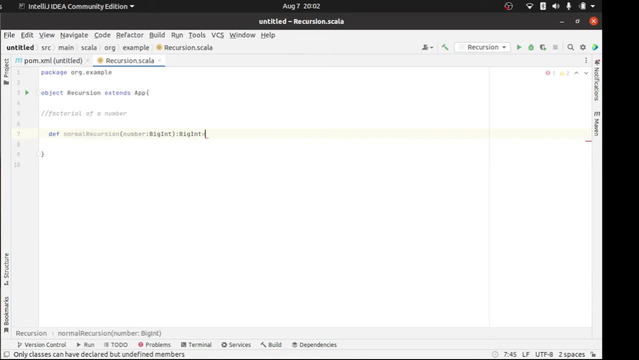 the upcoming section of this video because it will give you a much more better clarity why I have taken this big integer. so now I will be writing the normal regression function to factorial of a number for factorial of a number. so let's write the base condition like: if the number is less than one, then return. 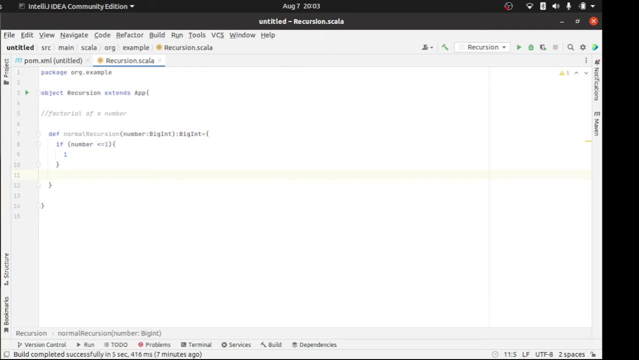 one otherwise, or else else return the number into and again calling the normal regression function, this time with number minus one. so let's print the value, that what is going to come. I'm keeping it as normal recursion function, normal regression function, and I'm calling the function with the very good number, that is five. 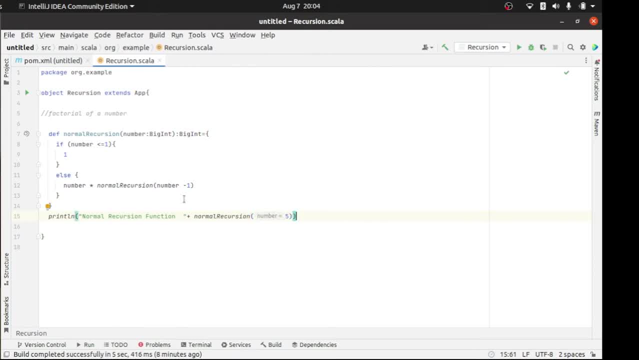 now let's run this application to see the output of the function. so we should run this application to see the output of the function. so now we are creating a function out of it for fetch error, so let's run this function out to find the value and then return the value, perform. 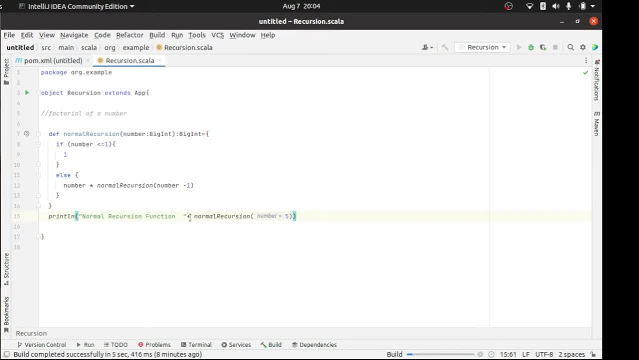 like this. so let's take this without Sportscard. so this action will return the reuse function. so before I say, before I do anything, we will toilet the function value and the value should come as 120. as you can see, the factorial of 5 is 120, so let's our id build. 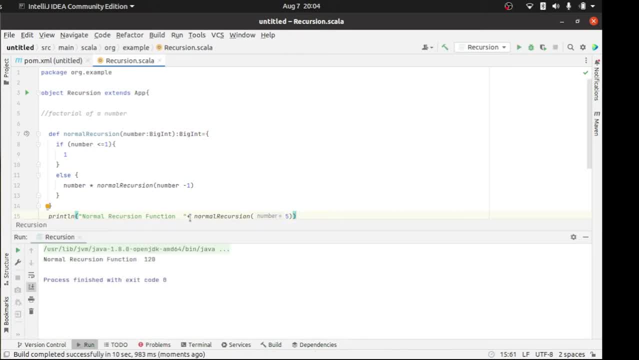 it and we have got our result as 120.. now you can see here our sign has come, and this sign is saying: the method normal recursion is recursive. so it is our recursive function, but it is not a tail recursive function, and i will explain you why later. then first write the tail recursion function. 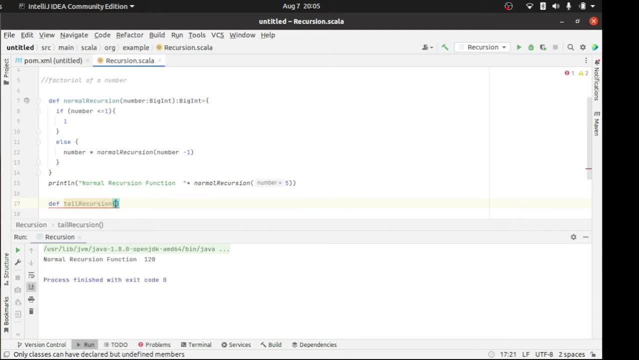 for the tail recursion function. one of the major, most important concept is that you have to make this recursion function as common. thanks for watching to always take a accumulator, because accumulator will store your result output and every time the accumulator will be changed and passed into the next. 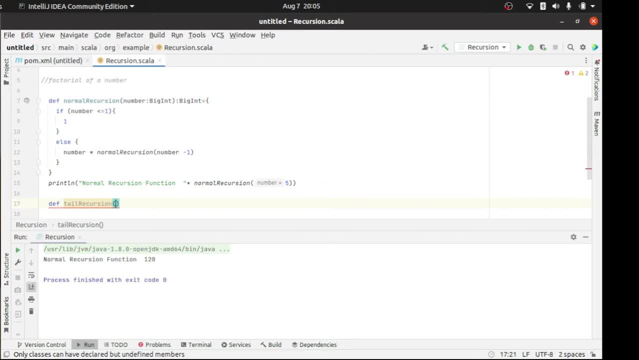 step. this is one of the major, important difference between the normal recursion and the tail recursion. so you will have to always take a number number, which is a big integer type, and also a accumulator, which will also be of a big integer type. why I am taking big integers, I will explain it later with 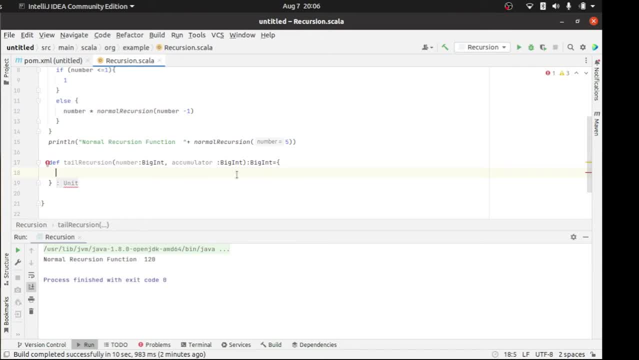 some big values. so now let's define our base scenario. if this number is less than or equals to one, then our function will return this accumulator. we will have to return the accumulator, not this time the number or one, because the accumulator will store the previous output values. so I am returning the. 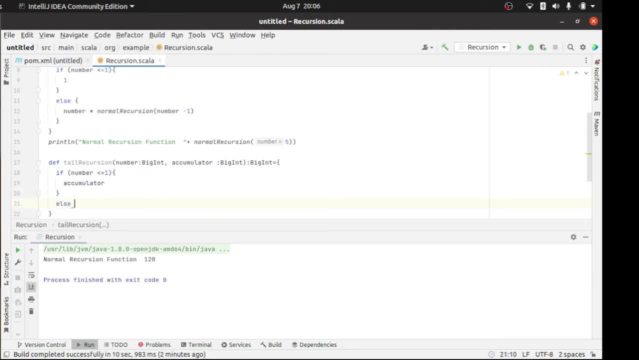 accumulator this time, and else I am calling again the tail recursion function with number minus one and accumulator into number. this is the major step here. you can see that the tail recursion function will be called with number minus one. I am decreasing the number with minus one and multiplying the. 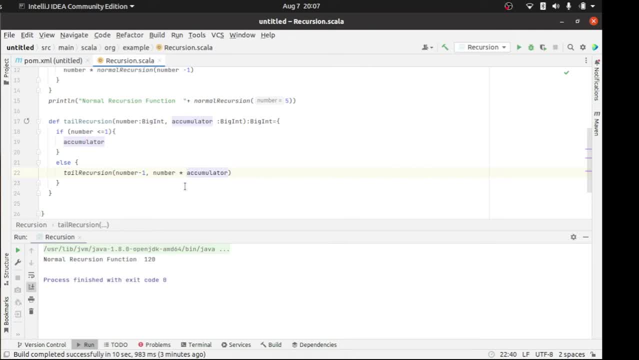 accumulator with the number and then again, in the next step, the accumulator will come here with the multiplied number. and the next step I'll be checking. if it is greater than one, then I will number minus one and number into accumulator. so this way we will be defining the factorial. 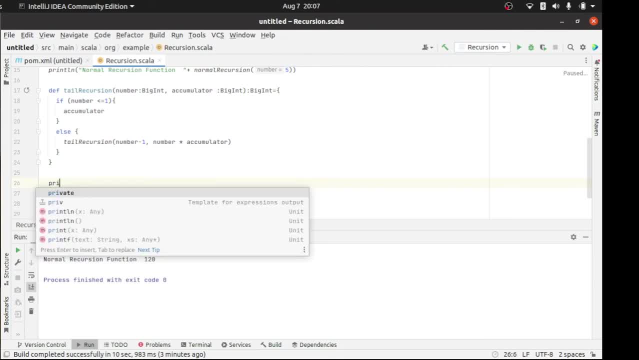 function. so here I am calling the printLn function to print our value. you, you, you tell output which will be again. we are seeing the tail recursion function with the number five and we will also have to pass accumulator for the factorial function. we will have to pass that accumulator function as one, the 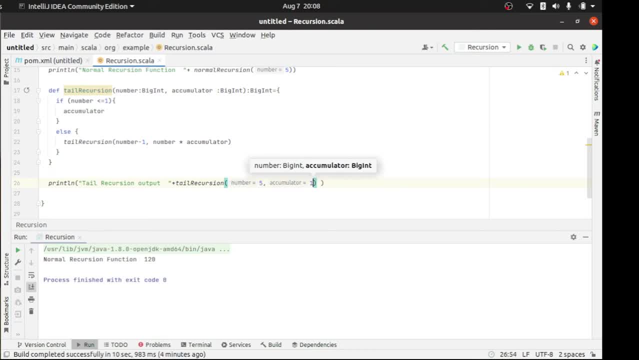 accumulator value as one, because if you multiply one with some function with with some numbers, it will return that number. for this factorial you have to take the accumulator as one. in your cases, you will come across some problems when you will solve the tail recursions. in that case you will have to take the 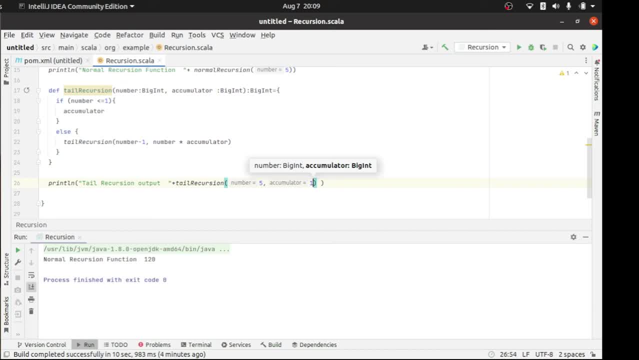 accumulators accordingly and it will come as a practice. so let's run our program and see what's the value. our compiler is compiling the output and let's see what is the output. yes, here you can see the two lines have been printed. the normal recursion function. 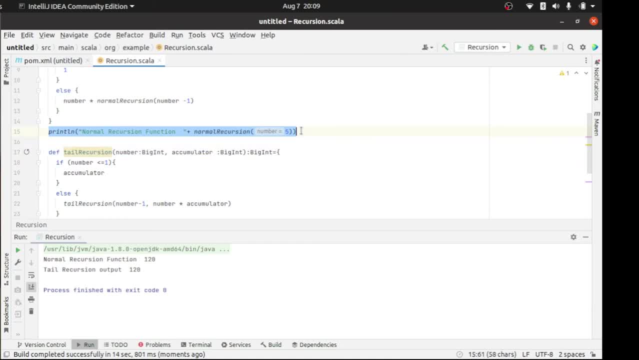 and the tail recursion function. let me just cut this line and paste it here so it will be helpful for you guys. so see what the two lines: a I am calling normal equation function with the value, with the number five and the tail efficient function with a number five, an accumulator, one, the accumulator. 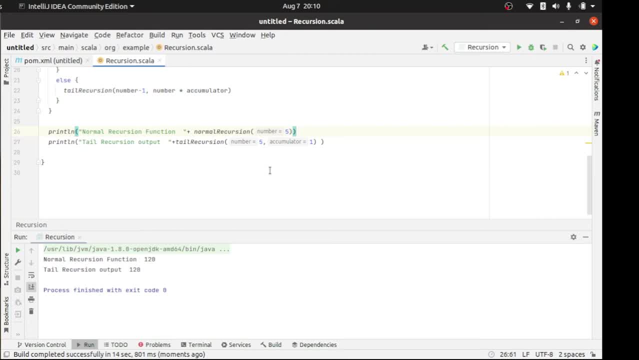 one is always given every tail equation function- and here's one of the major things thing- that already our Intel EJ ID has declares this method as an active tail recursive function. Here you can see the tail recursive word has come and it is a tail recursion function, which is particularly for Kela. 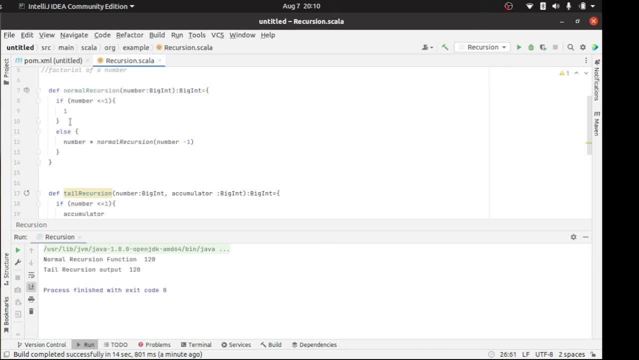 The method normal recursion is recursive, So this function is normal recursion function and this function is a tail recursion function. Now here see the catch that why the tail recursion is very much preferred option for a large amount of data. So now I am going to. 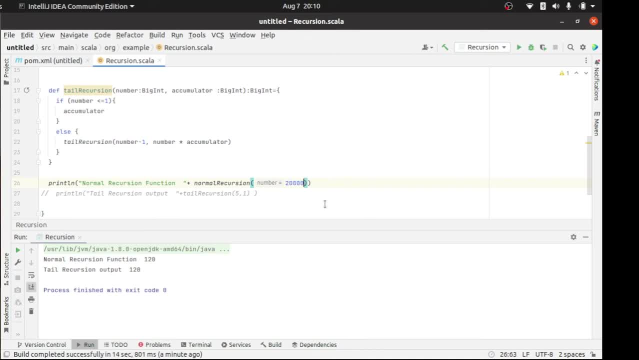 give a large value of factorial. Let's see the 20,000.. 20,000 is a very big number for a factorial. Here you can see the multi-million digits will come in our screen. but let's see what is the response of this program. 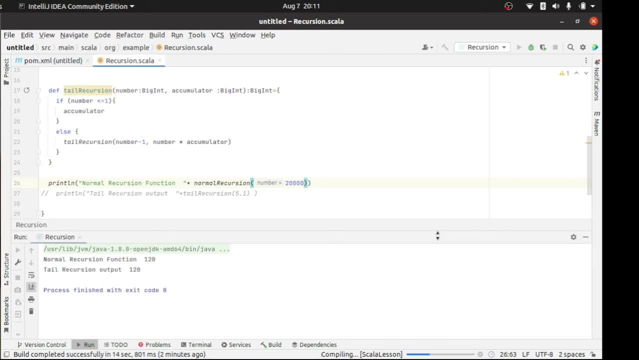 So I have given the compiler to build the project and to run. So let's see what is the output. Here you can see the recursion function has been processed. finish with exit code one. The exit code one here comes because our stack memory has been completely full. Normal recursion function. 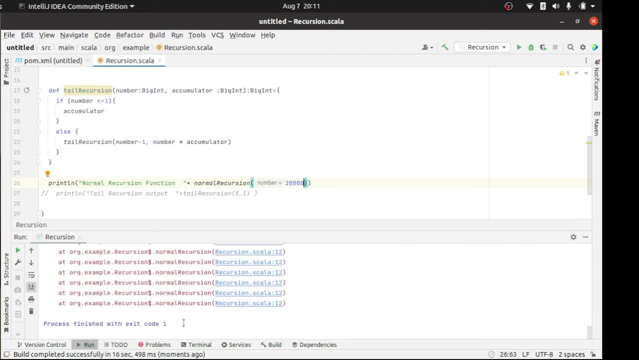 will be completely full, but the recursion function will not be fully full. The recursion function will be completely full, but the recursion function will not be fully full. The recursion function will call the recursion again, again, again and again and it will give you many more objects and it will absolutely fill up your memory and that's why this normal recursion. 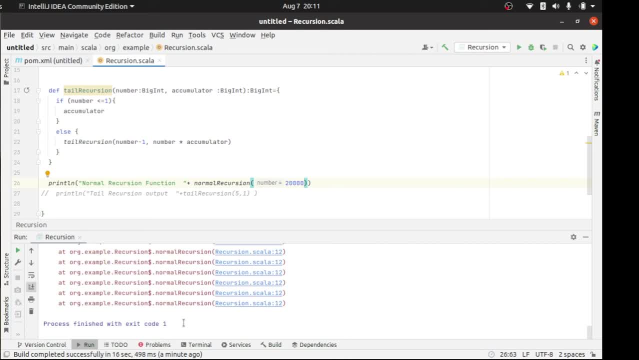 function is never preferred for a large set of data because that case your memory will be totally full. That's why this recursion is not preferred for large values. Now, if I comment this line and run this tail recursion line with the same value of twenty thousand and our accumulator will remain as one. So let's see what is the output. 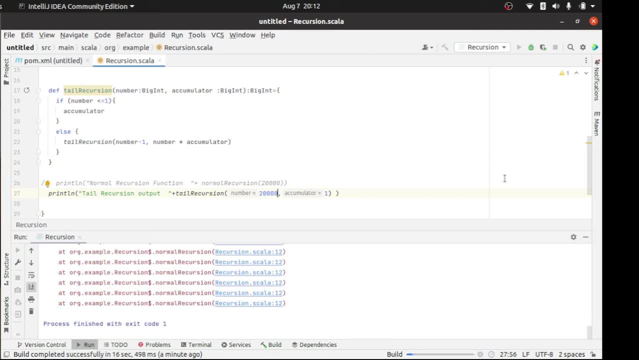 Can our compiler generate the output or it will fail again. So our compiler is working and voila, it has given a value of something very large, but it has given a value. Here you can see the very much big value has been given and here you can see that it's out. 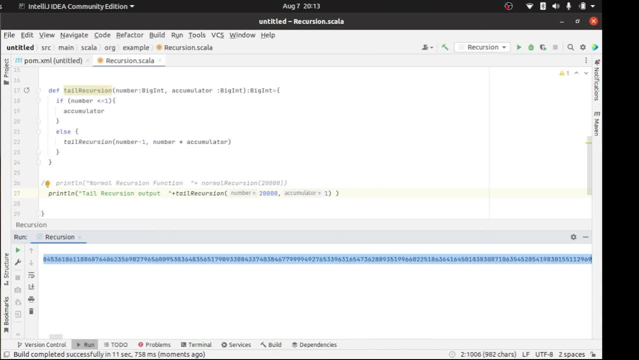 of the ranges of the screen, but still our compiler has managed to compile this program and run it so successfully. So why this happened? So, the tail recursion function. So basically, what is the tail recursion function? And also one of the major, important thing you can also give. 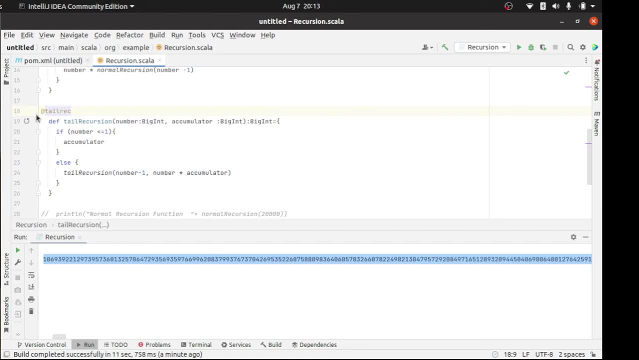 this annotation as tail-rect to to let people know that this is a tail recursion function, because the tail recursion function is somehow much more efficient, more preferred in a big data environment and are very good resources where distributed programming has been done, because a very large amount of values 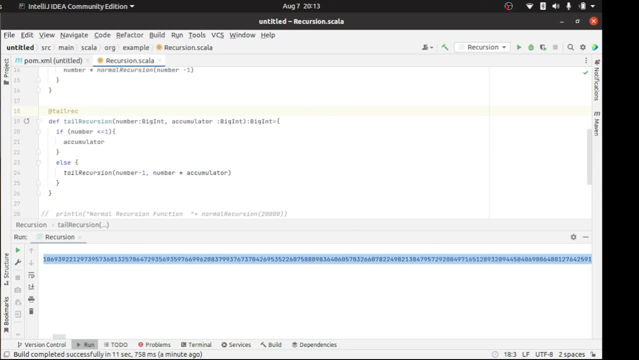 can be handled by this tail recursion function. so this tail recursion annotation is much more preferred and you can let your people know that this is a tail recursion function with this annotation. so now come into the point that, why the tail recursion has handled our 20,000 factorial problem, but our 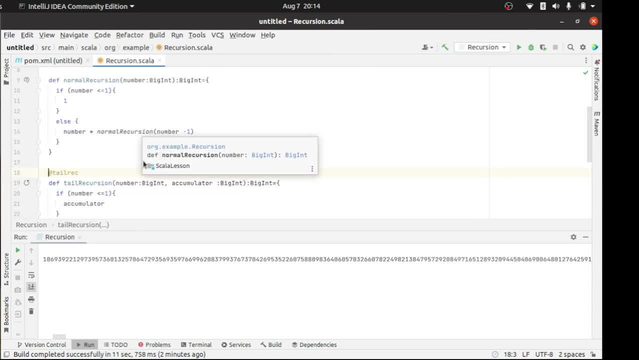 normal recursion could not. so the tail recursion function will come. so our scalar compiler will compile the program. if it is saying that our tail, our function, is a tail recursion function, then it will internally convert that recursion in a loop and a looping function will work on the data, not a normal recursion function.